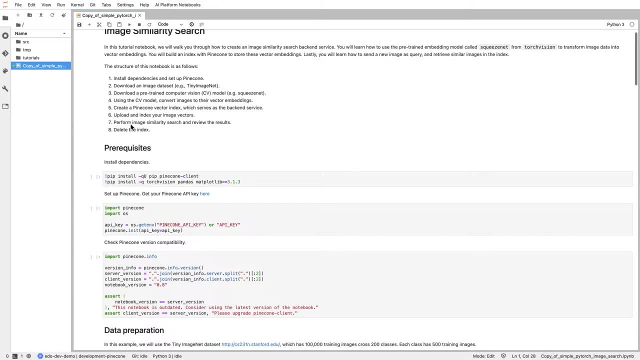 We'll use that to actually transform the images to vectors. We'll create an index, We'll upload and index all the images in vector form to Pinecone and then we'll perform some queries, look at results and delete the index. So without further ado, 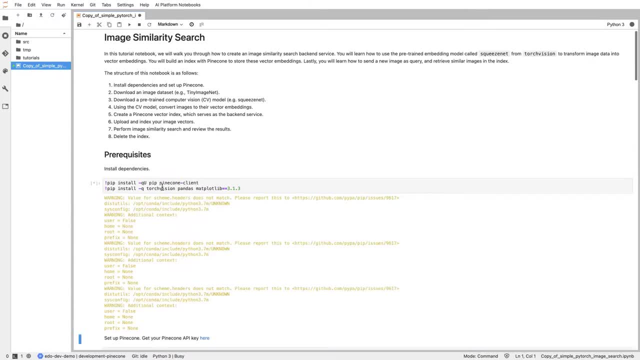 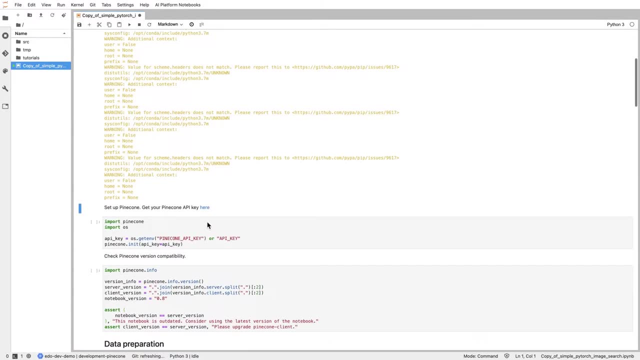 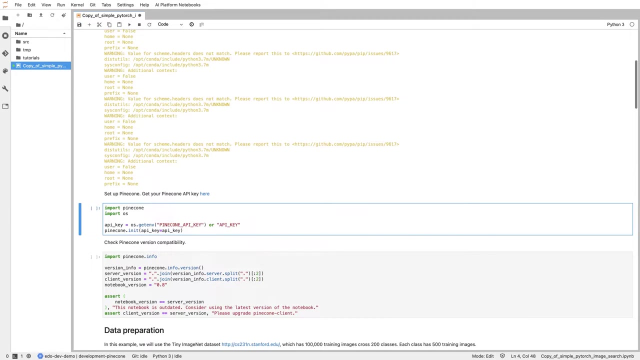 let's install some dependencies. Here I'm installing the Python client, I'm upgrading my pip install just in case. I'm installing TorchVision, Pandas and MatlockLib for showing some stuff That is done Here. I have to put in my API key, which I have, and so I'll copy it. 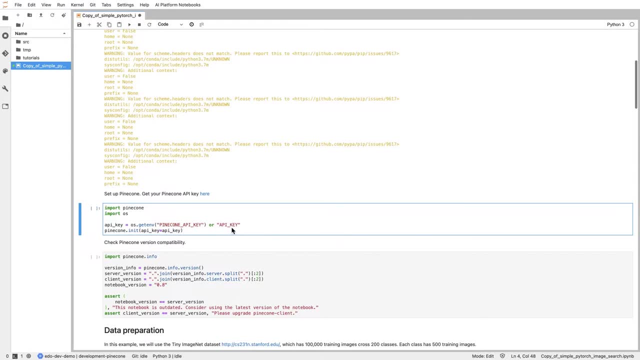 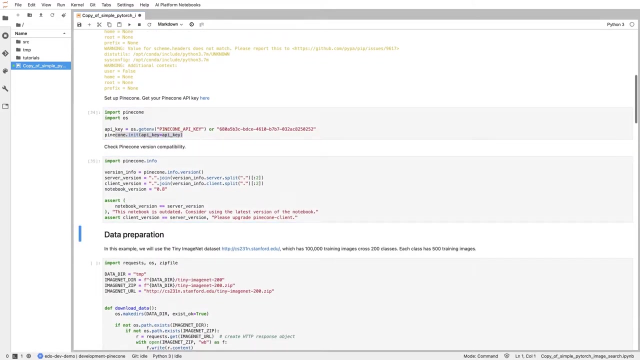 Give me one second. Here it is, And so now I have imported Pinecone and I've initialized my client and I can run now as an authorized user Here. I'm just confirming that the versions match. You don't have to do it every time. 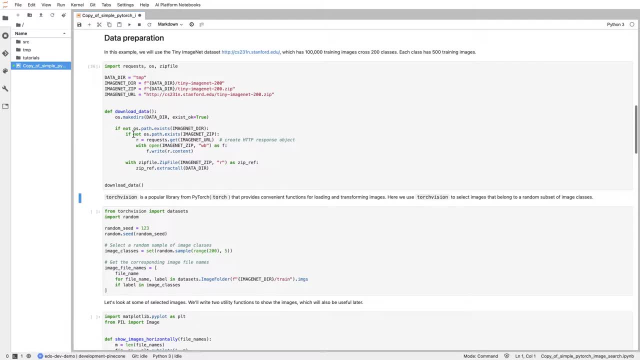 Here I'm downloading Tiny ImageNet. This is not a very large data set and the GCP connection is very fast, And so I have- I think actually I've already- pre-downloaded those to this instance, and so that is pretty quick. 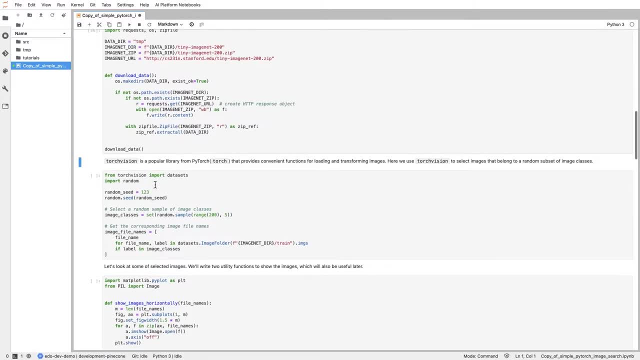 It just checks that the files are there, but it usually takes, you know, maybe 10,, 20, 30 seconds Here. now that I have the data out, I'm going to go ahead and install it. I'm going to go ahead and install it. 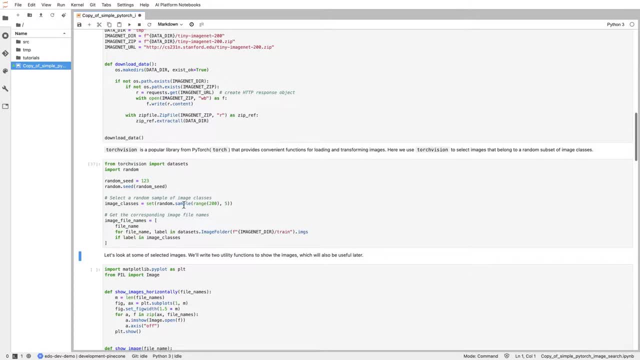 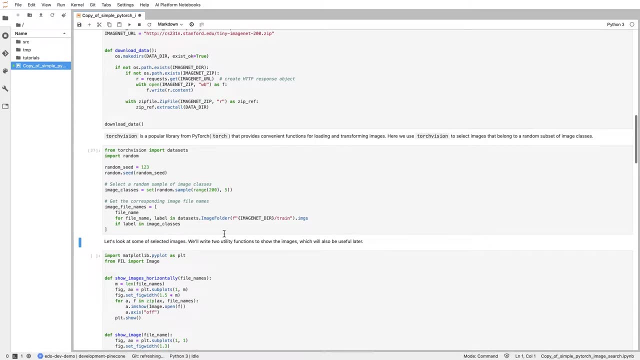 Here. now that I have the data out, I'm going to go ahead and install it. I can use TorchVision. It has a nice utility that lets me iterate over the folder structure and create a flat list of data of file names and labels based on the folder structure. 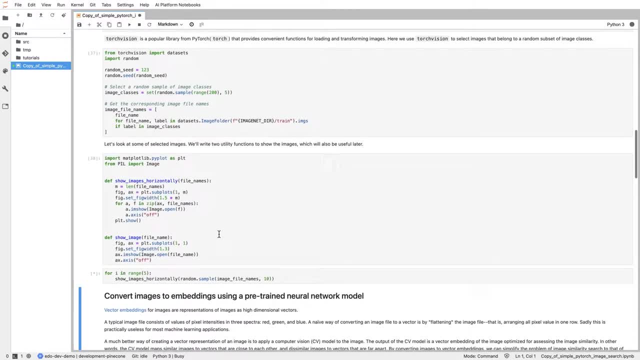 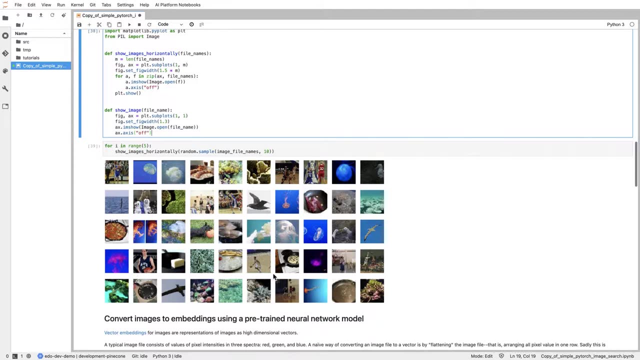 And now we can look at those images, And so this is: these are just utility functions that print images to the screen, and this is, you know, an image not unlike the one we saw before, Just a collection of those, like some food, some basketball. 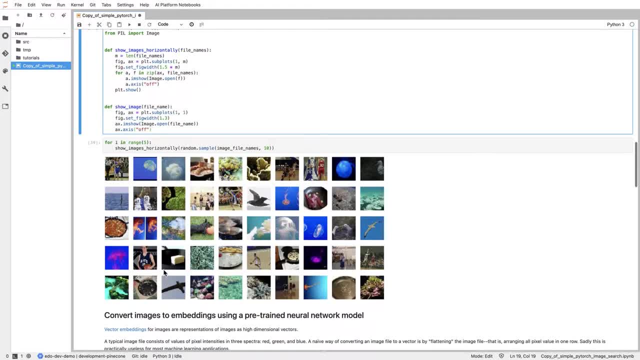 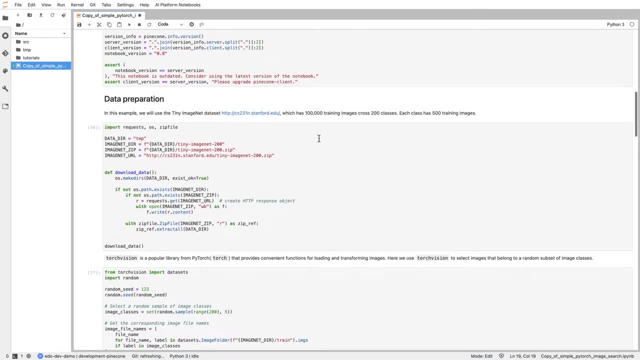 some corals and so on. So this is the sample from our data set. We have- I maybe did not mention it, the data set is 200, sorry- 100,000 training images across 200 classes. you know, 500 images from each class. 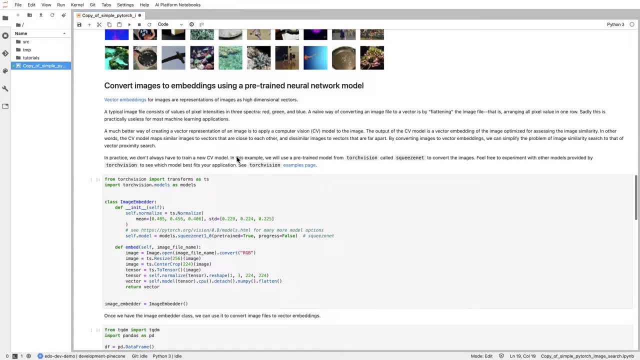 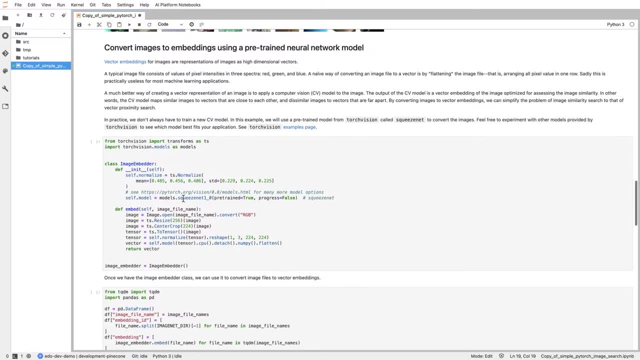 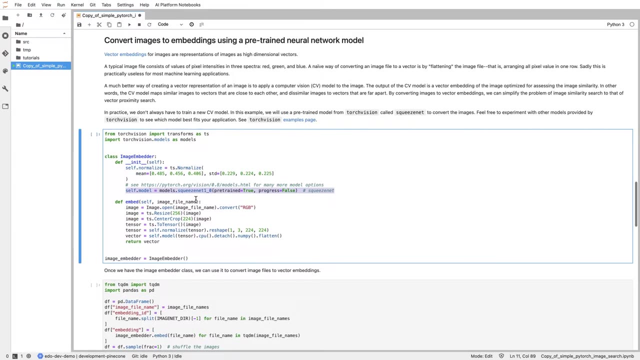 Now we need to create a model that transforms images to their embeddings, their vectors. To that we're using, we're using PyTorch and, specifically inside with PyTorch, we'll use PyTorch to download pre-trained version of SqueezeNet. 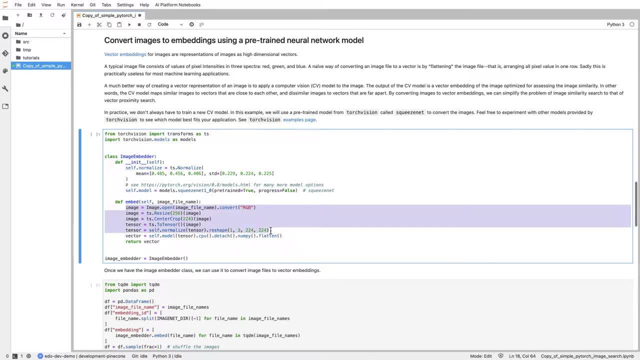 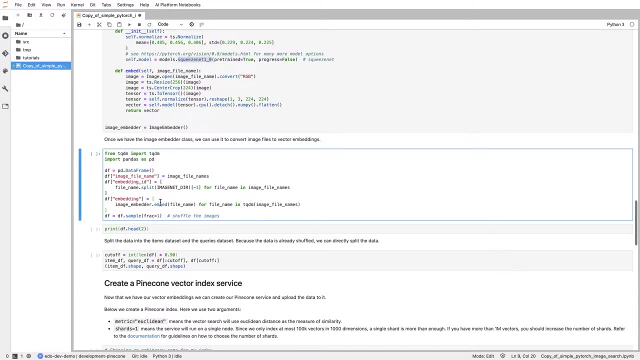 For each image, we'll perform some rudimentary normalization and then apply the model here, And so this class now downloaded this model and created a class that is able to transform images. Now I need to actually transform the images, And that takes a few, maybe like a minute or two. 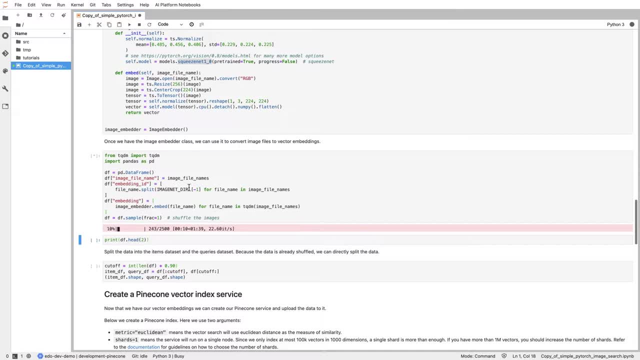 Note that this instance needs to now apply this model for every image in my data and create this vector embedding. I note that it's possible to actually give Pinecone the models themselves and have Pinecone be in charge of this step, But it's more involved and I think it's outside of the scope of this demo. 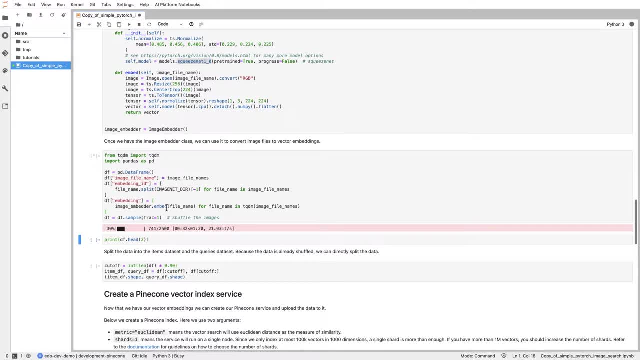 And I think kind of the main idea is, more is already shown through PyTorch, So we'll have a lot of data that we can use to already converting the vectors and uploading the actual vectors to Pinecone. We should be done with this fairly quickly. 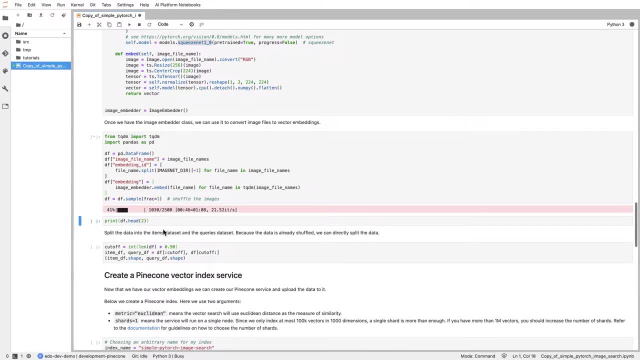 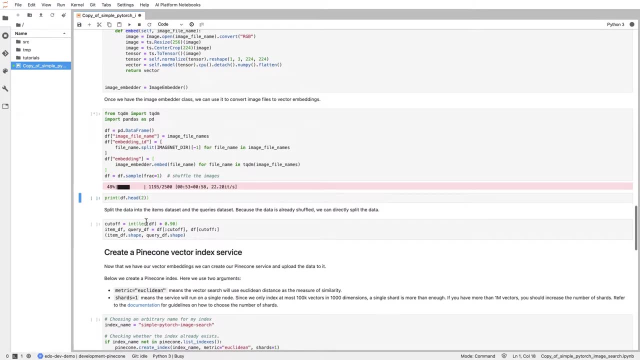 Here. we're only using 2,500 images for this example, What we'll do later. while this is running, we will split the data as 90, 10.. So what is like 2,250.. Am I doing this correctly? 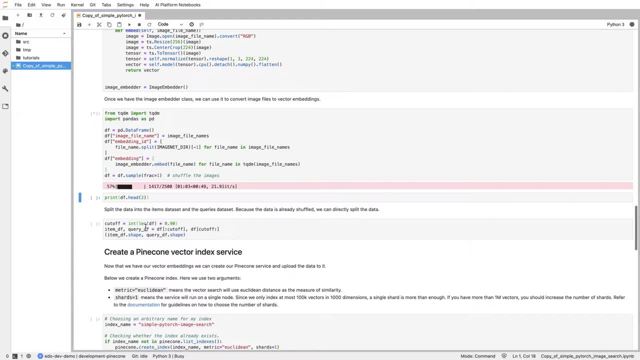 Points. images are going to be in my corpus, So these are going to be using my data And I'm going to use my data. So these are going to be using my data And I'm going to use my data. 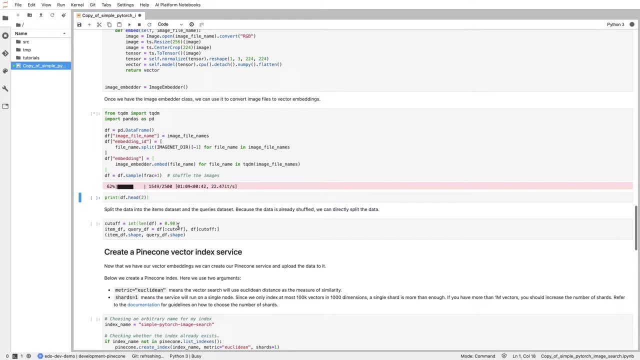 So these are going to be using my data, So these are going to be using my data. So these are going to be using my data And I'm going to use 250 images as queries. Okay, So this is what this split does. 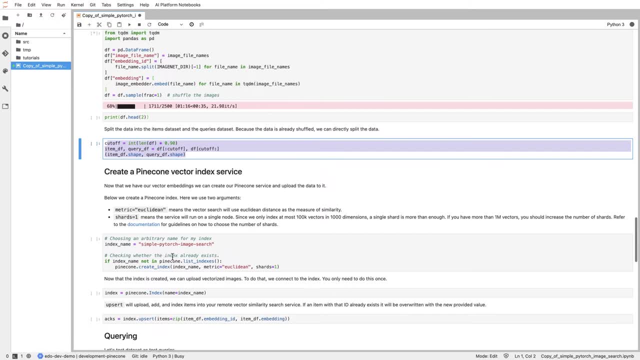 We'll run that in a second And then we'll create an index, And so here I'm just naming my index. This is the first time I'm actually using Pinecone. I'm just creating a string. This is the name of my index. 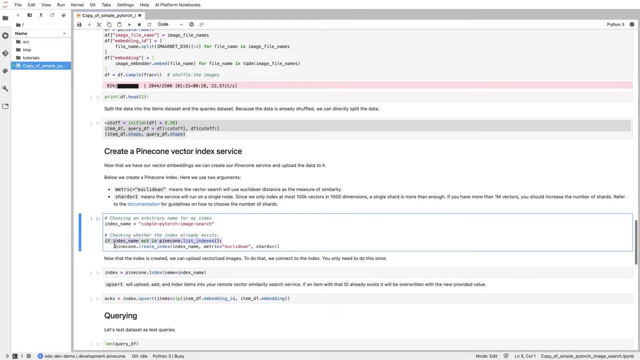 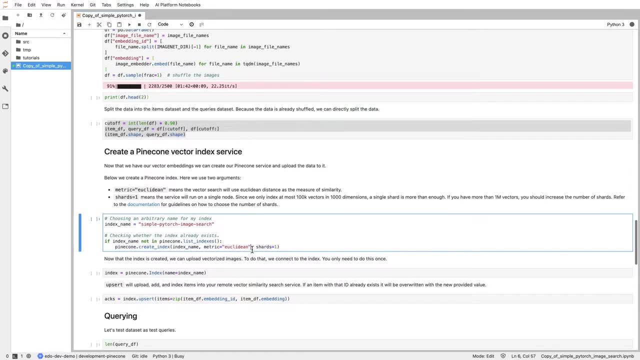 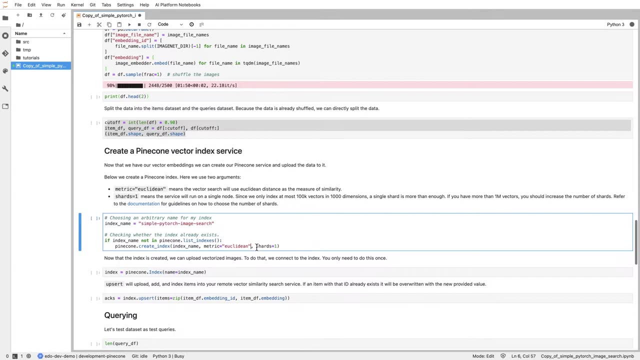 And here I'm creating the index. I'm giving Pinecone the name of the index. Here it says you should use Euclidean distance as the measure of similarity. So closer means more similar And it's a relatively small index. 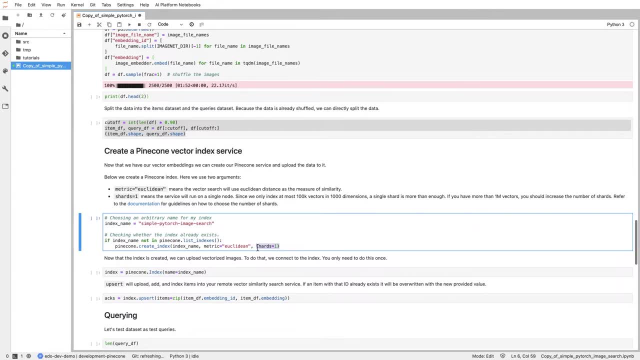 And so I can use one shard. You can use more shards if your data is larger. You can use replication if you need a higher QPS, and so on. We're not going to go into that here, So this cell is now finished. 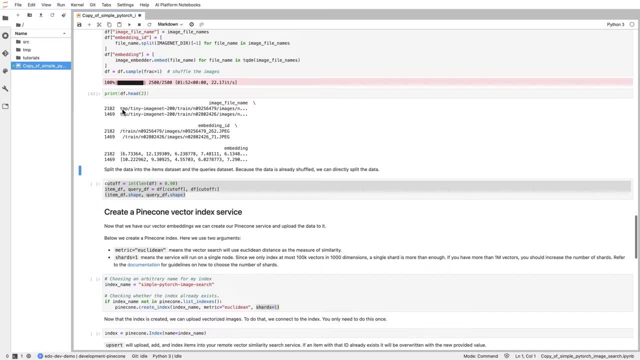 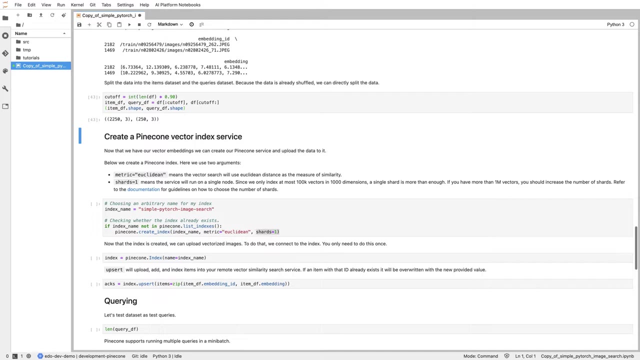 I can now run this. Just look at my data frame. My IDs are just the names of the files on my Local hard drive, and the embeddings are these vectors. And so now I can split the data and let me create the Pinecone service. 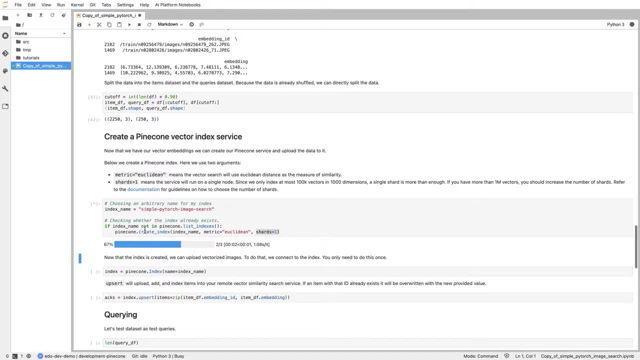 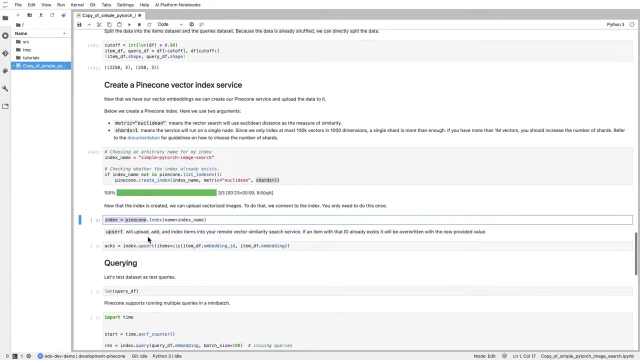 This should take only a few seconds, All right. So now we have a managed service, a vector index, and I'm going to run the Pinecone side. This is a remote service, of course, This isn't happening on this machine. 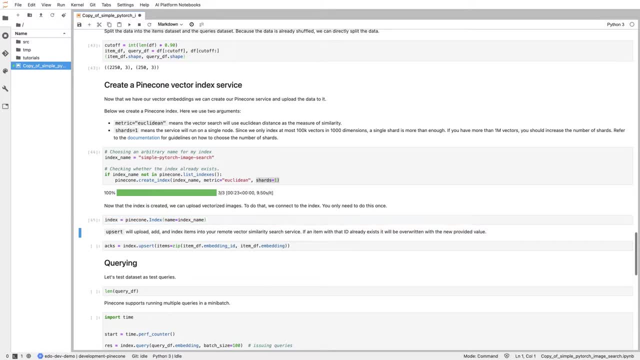 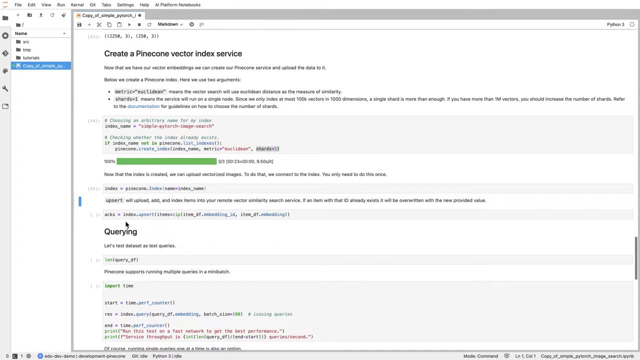 And so for me to connect to it, I have to create a connection, which I'll just call index. Mind you, the index itself is again as a channel, as a connection. It isn't the object itself, It isn't the index itself. 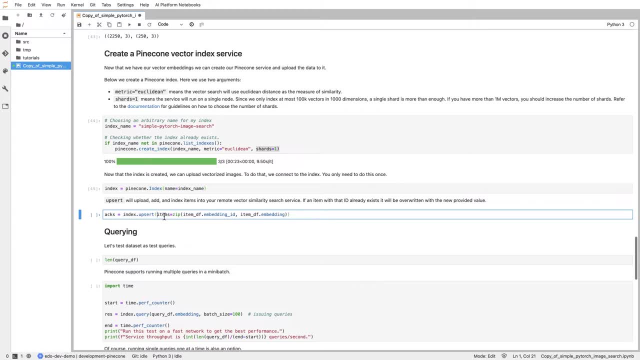 And here I'm up-serting. So look, I'm creating indexupcert And what it gets is a list of tuples being the IDs as the first object, the first item in the tuple, and the vector as the second item. 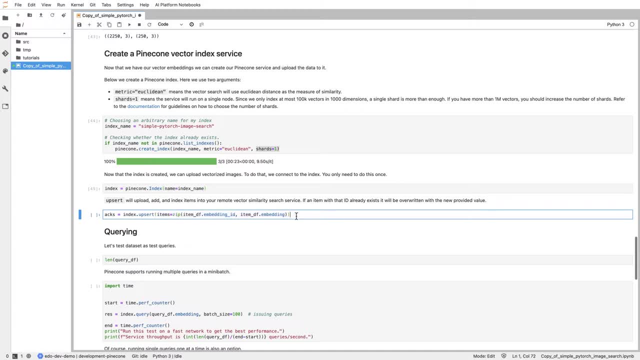 And this is just an iterator over those. So here I'm running the upcert. Note that it was incredibly fast. So Pinecone already ingested and indexed 2,250 vector embeddings corresponding to my images and their corresponding IDs. 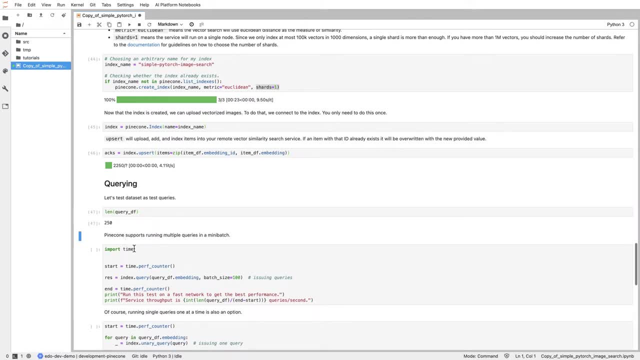 Look, now I have 250 queries that I would like to issue Here. I'm going to run those queries as a backup, So I'm going to run this batch. This batch is of size 100.. So that would be three query requests. 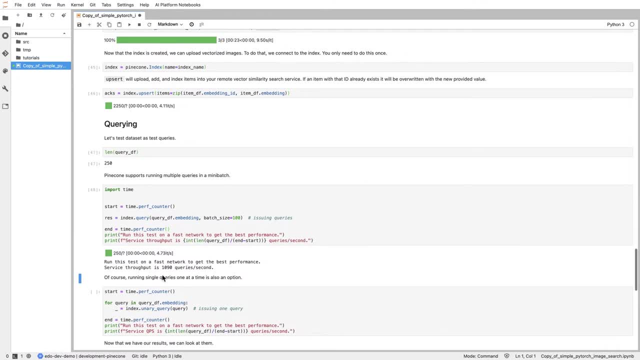 I'll time it just so we can see what we get out of it. And here I'm getting a throughput of about 1,000 items per second, 1,000 queries per second. This I want to stress that this is highly dependent. 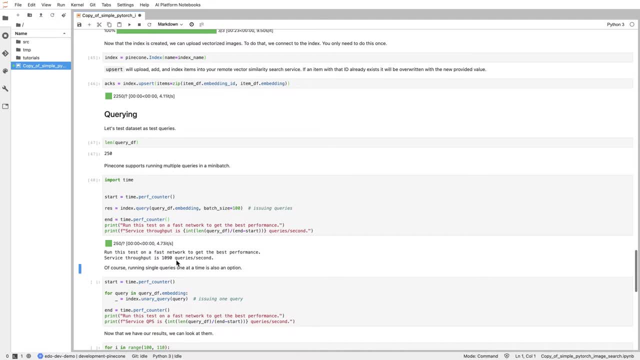 on the network you're operating from. If you're in some place random on the cloud, it might be that it might be slightly lower. it might be slightly higher If you're operating on a Google Colab or some less performant environment. 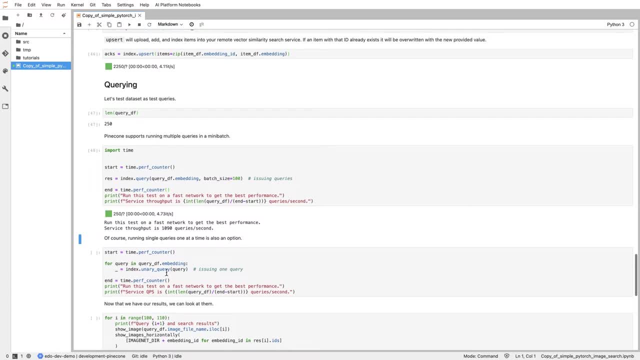 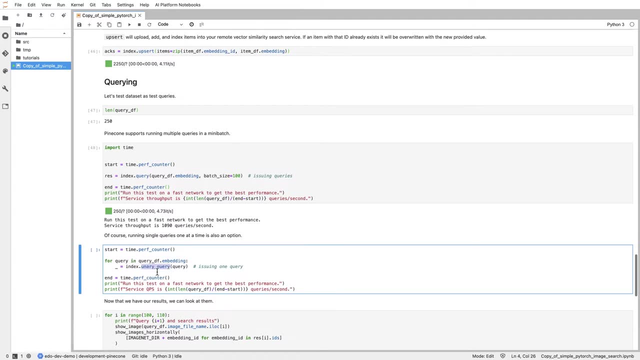 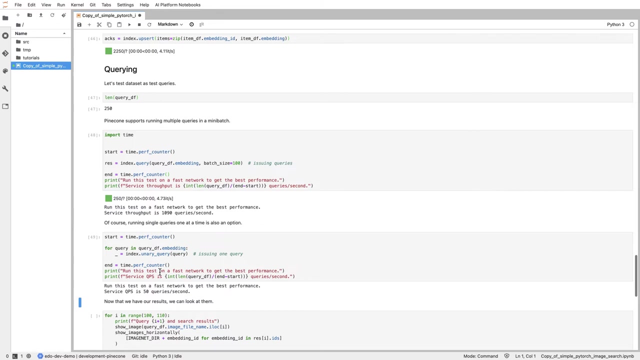 it might be lower, And on your laptop at home this would be quite significantly lower. Most services actually call to what's called unity calls, And so these do queries one by one, And that is, of course, significantly slower because this is. 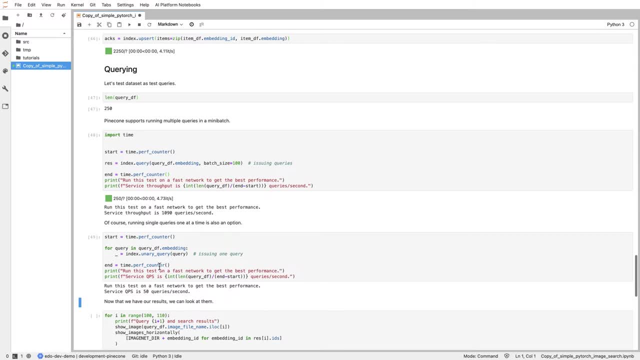 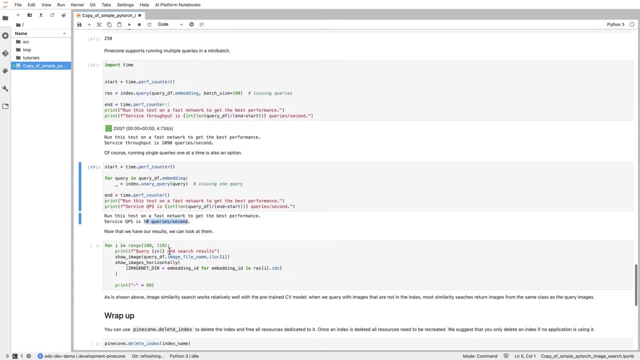 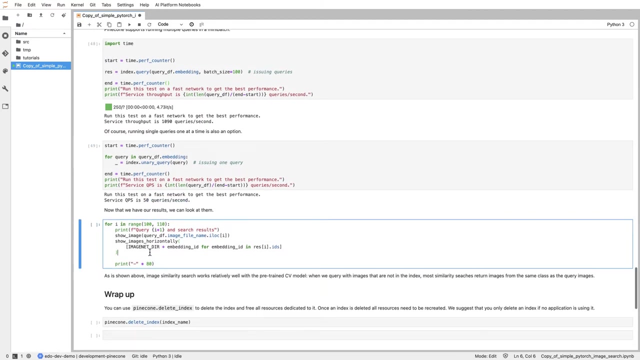 this is not batch, and so I actually have to do a round trip of communication for every query. We see that we only get about 50 queries per second in this setting. Finally, it's time to actually look at the results. To do that, we'll just print the relevant queries. 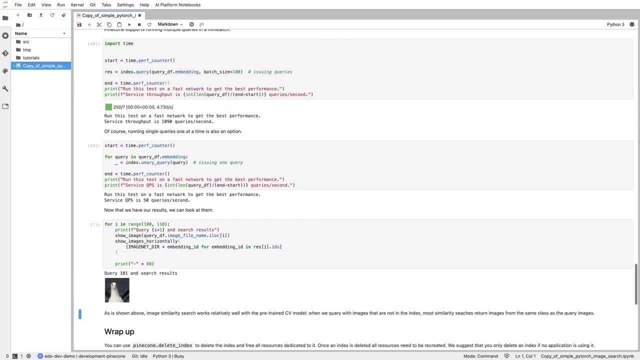 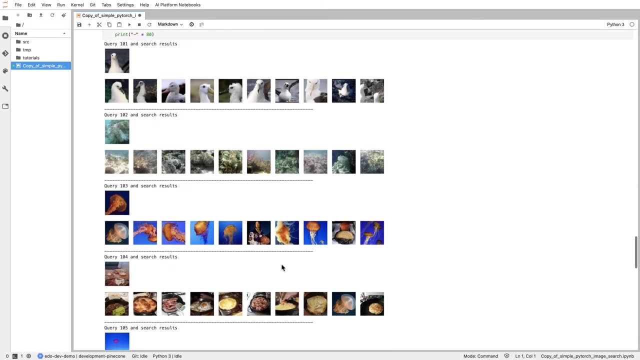 and then the images corresponding to the result set. And so, for gulls, we get most mainly gulls. For corals, we get mostly corals. This is, you know, jellyfish food, et cetera. 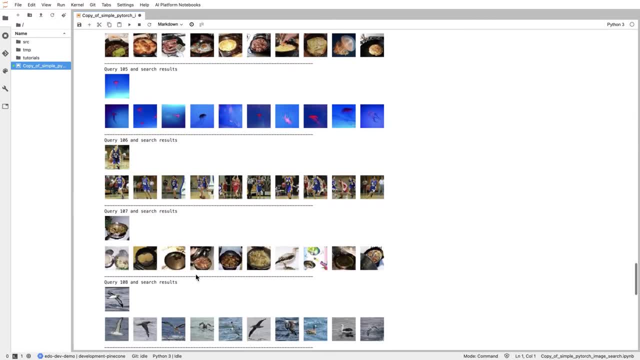 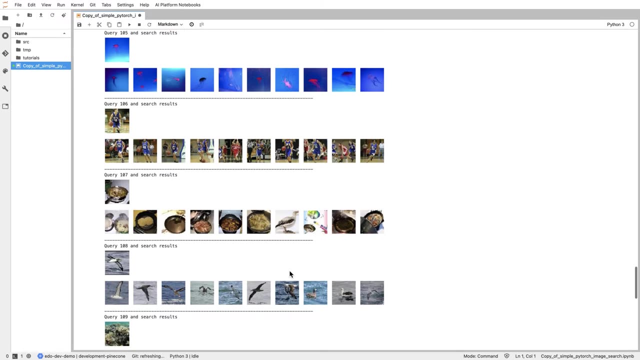 I'm sure I can find somewhere where this isn't perfect. Yeah, here for some. something frying in a pan. you get this, what seems to be a taxidermied bird, Or is it alive, I don't know. Anyway, so this. these are results for image search. 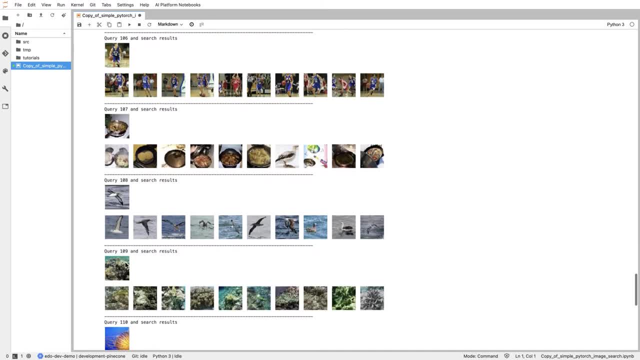 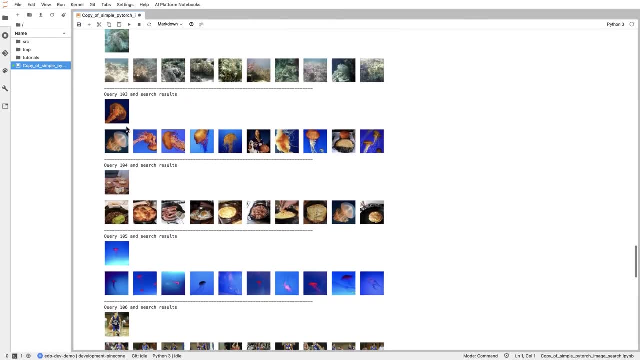 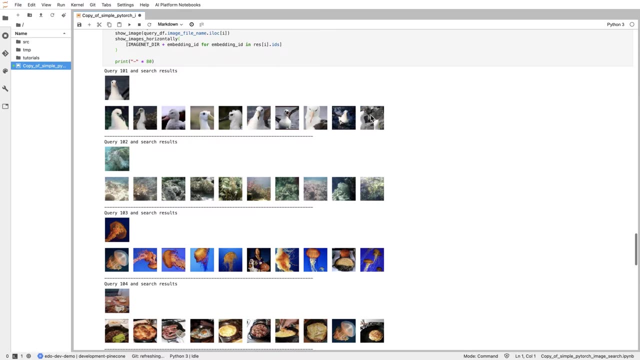 Note that this, some of these images have, you know, this image of this image of a gull, for example, The first one is very different than this last image of a gull, And so the comparison isn't done pixel-wise. 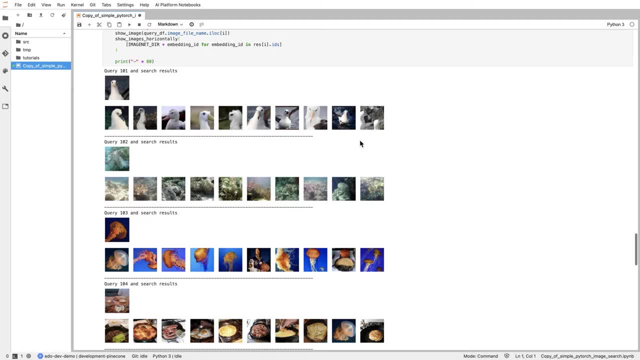 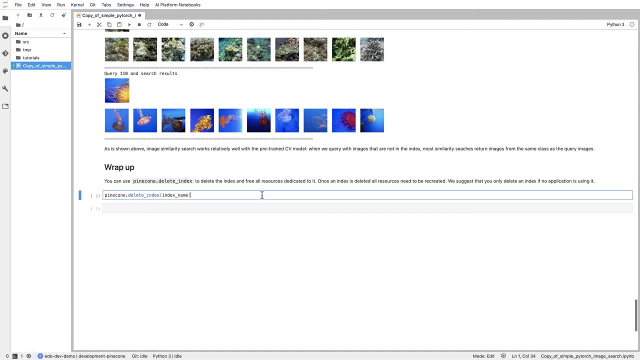 It's done- a much deeper semantic level for the comparison of those images. Finally, when I'm done with my service, obviously if this is running in production, I would leave that on. If this is, if this is just a tutorial for me and I'm done, I can just delete the index. 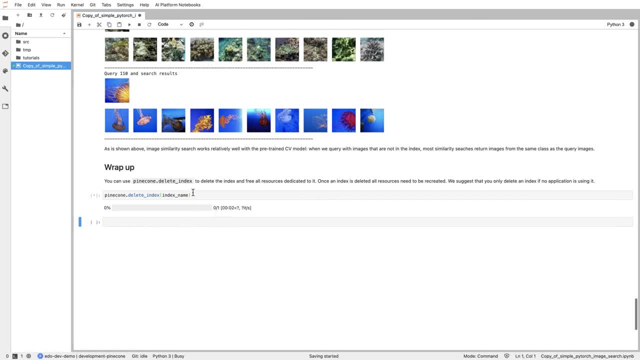 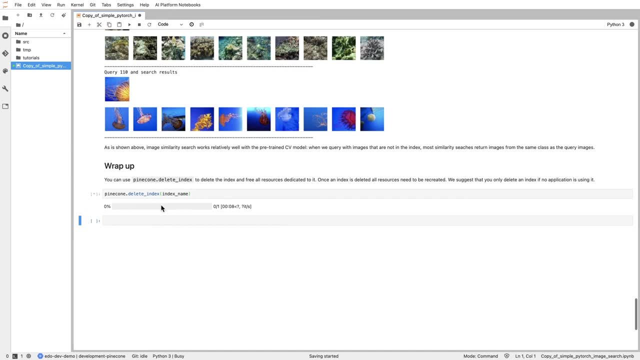 and free all the resources associated with it, And once I'm done with doing that, I don't I'm not using any resources on the on the Pinecone side and there's no service waiting to be answering questions, answering queries. That is it. 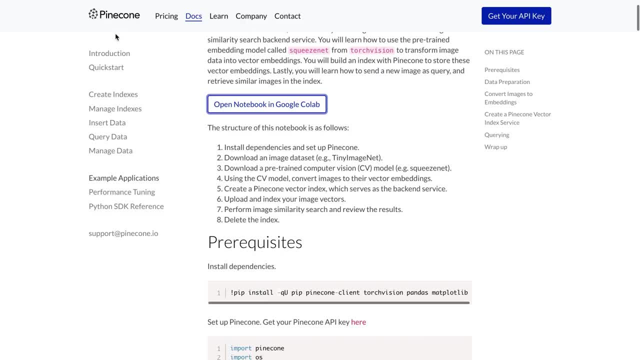 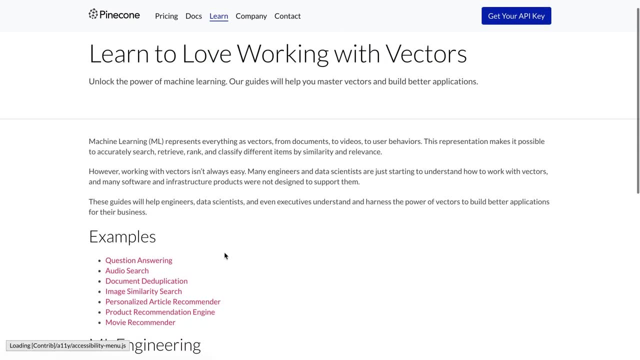 Thank you very much. I you know. I suggest you go to Pineconeio and look at the examples and tutorials. I'm sure you'll find something that you would like to try to do. Thank you so much.